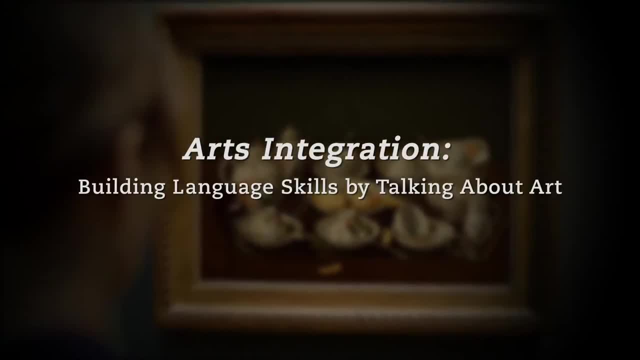 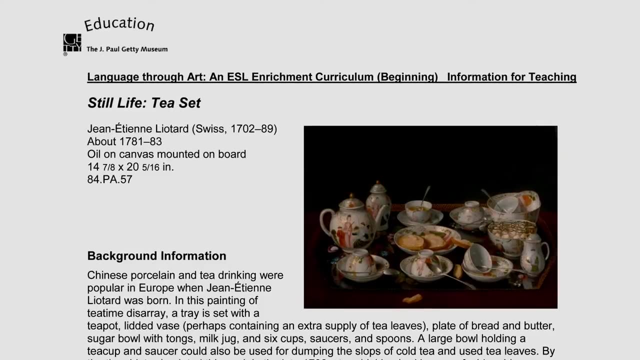 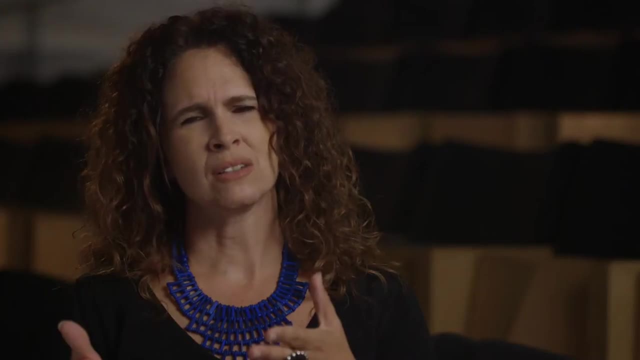 we were teaching the lesson to our students. This lesson really focused on teaching prepositional phrases through art. It was targeted towards EL students because that is an area that EL students have a lot of difficulty with. Rather than saying I'm standing on the rug, they 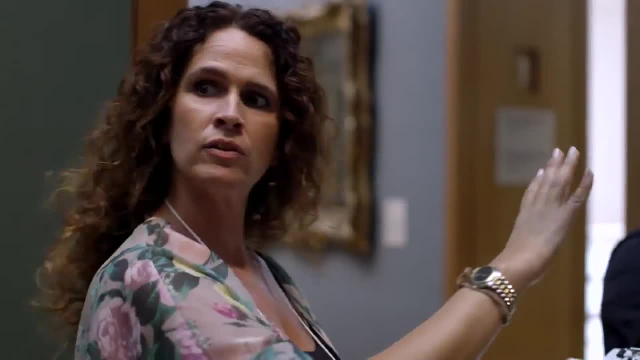 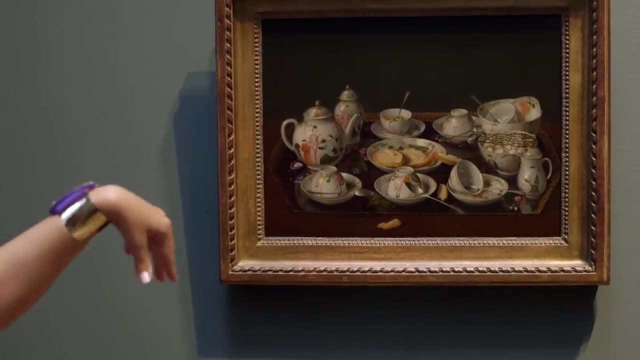 would say I'm standing in the rug. This was a lesson that really lent itself beautifully to teaching prepositions. I want you to look at the painting, ok, and tell me what you see. Yes, Teapots, Teapot, Good. 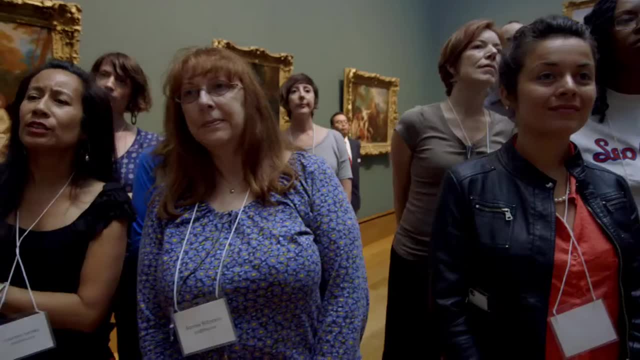 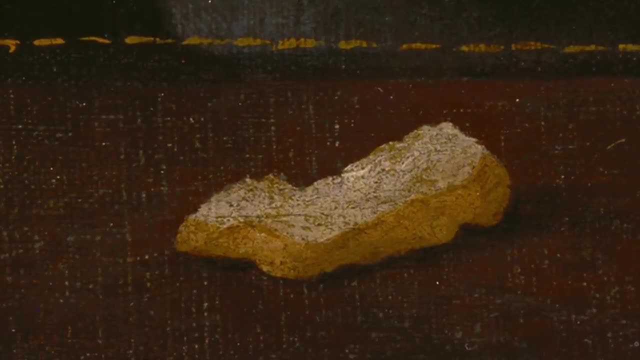 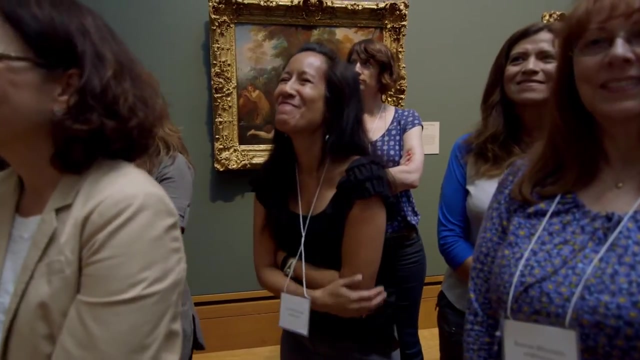 Teaspoon, Teaspoons. Very good, There is one piece of food all by itself. It's not even on the tray Right here. I think it's important for the teachers to experience the professional development as if they were the students, because when you are teaching the lesson, you are not. 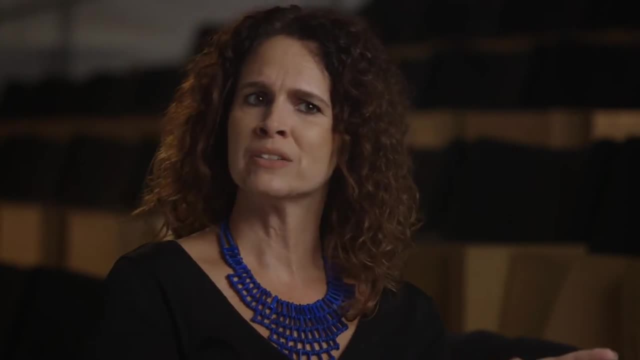 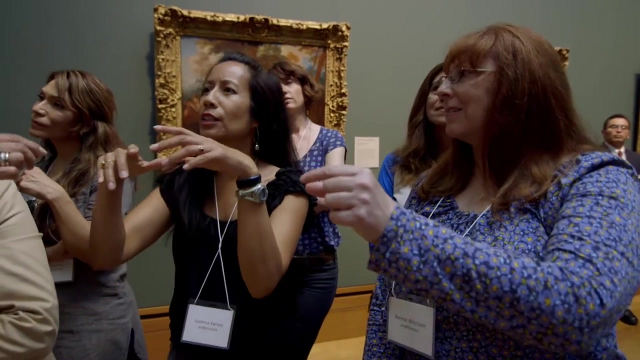 You are the students, You are the ones that do these particular things, lesson you remember. oh, I didn't quite understand that, so let me break it down a little bit more, or I think I could add on to this part here And you're able to put a little bit more of. 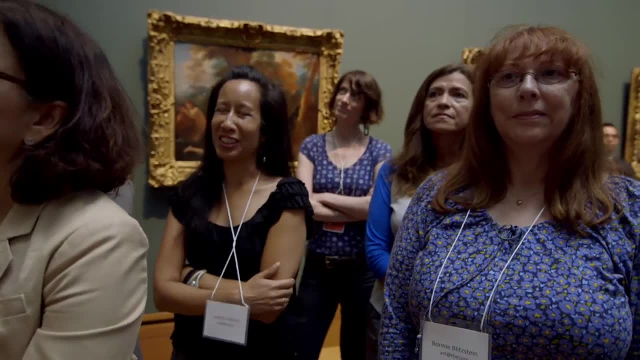 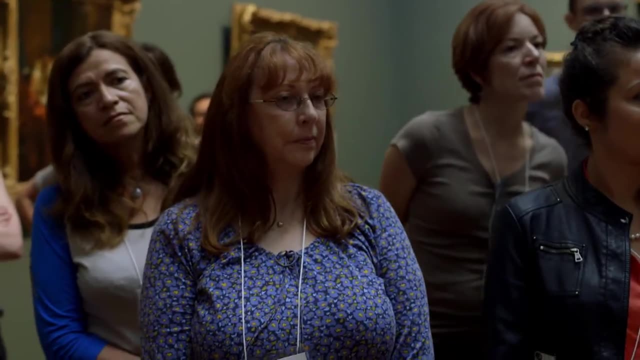 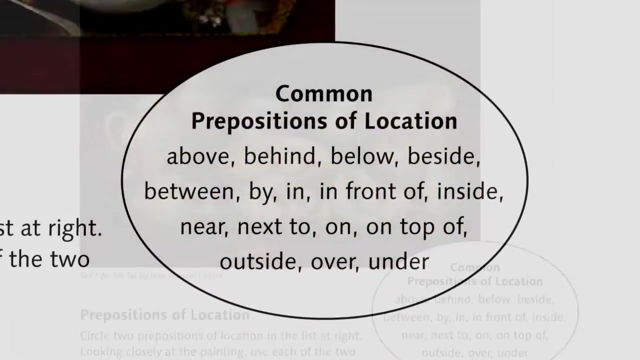 whatever your students need into the lesson. Now, this would be a good time, I think, to introduce some of the pieces that the children didn't mention, So like the creamer, and From there we started using the worksheet that went along with the lesson. looking at the. 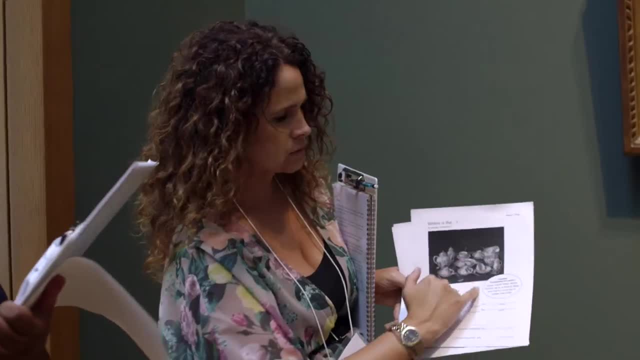 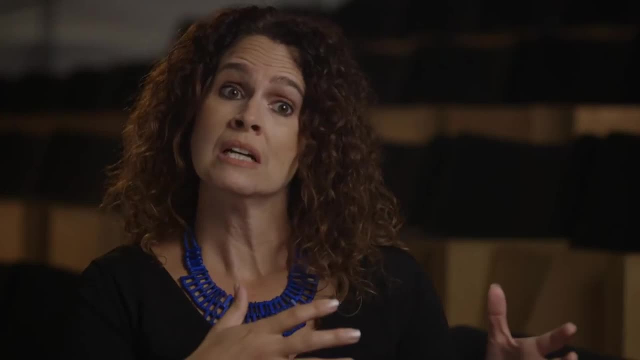 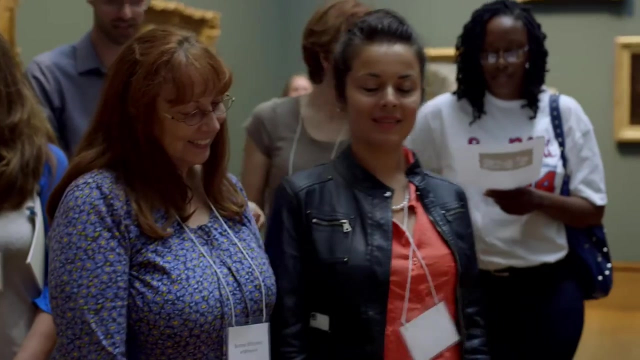 prepositions that they can use in describing what they saw in the artwork. First, we had the participants actually use each other to see what a preposition was In your partners. I want you to stand beside your partner. Beside is one of our prepositions. Now, have somebody stand behind. 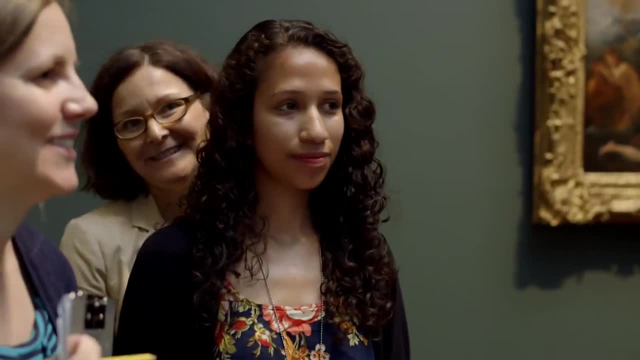 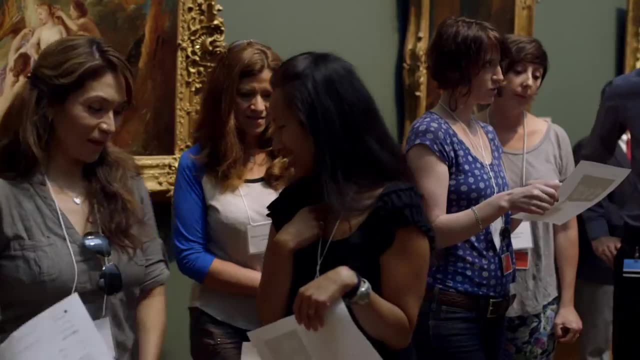 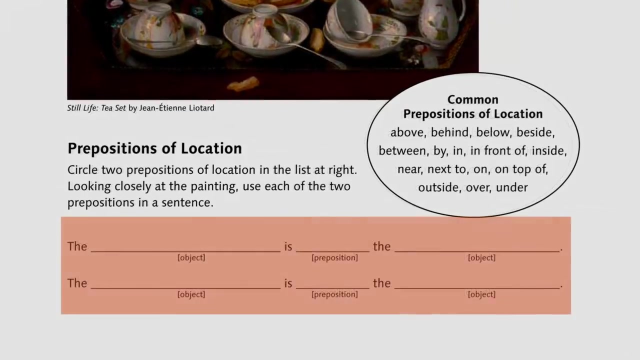 We weren't wanting them to see. well, oh, if I am behind someone, I have something in front of me, You know. so Then, after we had them actually move around, we had them look at the sheet and there were a couple of sentence frames on that sheet. A sentence frame is a guide for the 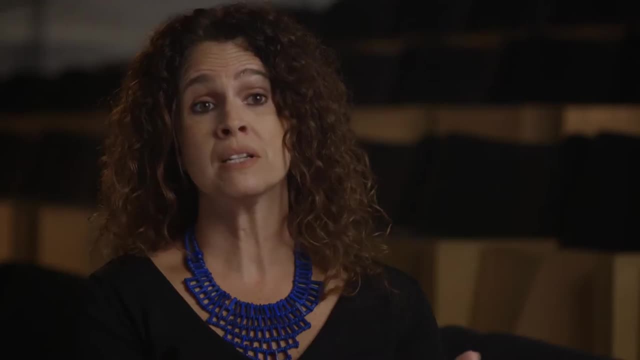 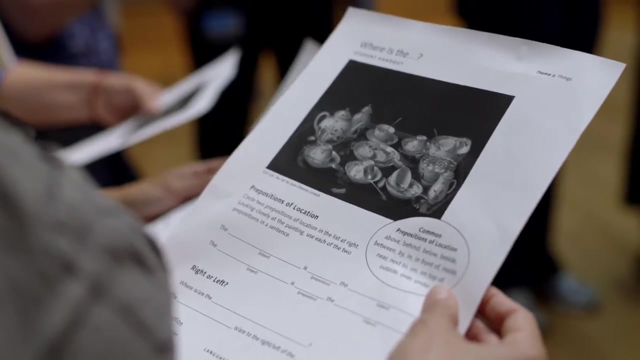 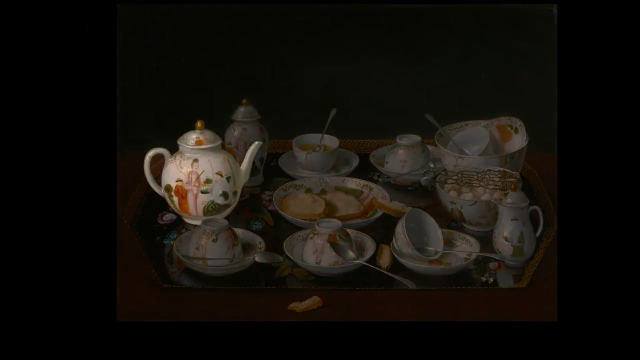 students in order to form a sentence. You know, depending on the level of English that the children come in with, they may need that. Once they feel more confident, they don't need to use it anymore. See if you can complete the sentence frames that are there. For example, the teapot. 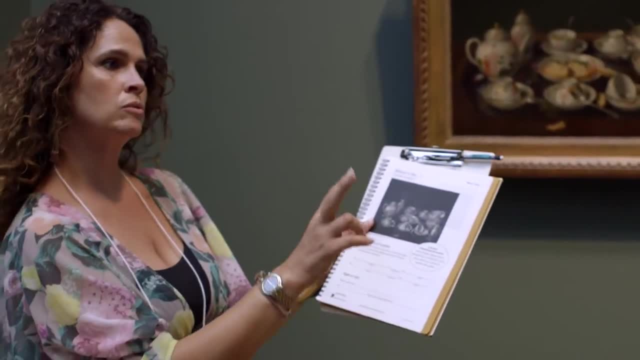 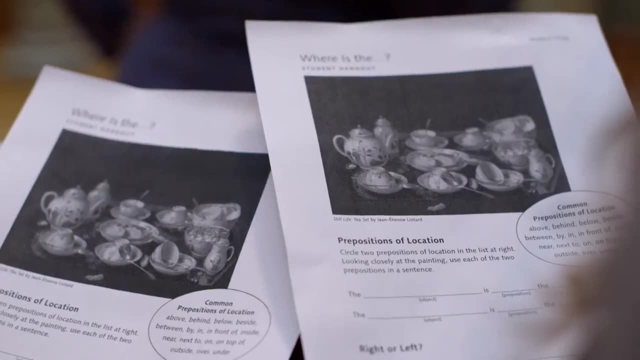 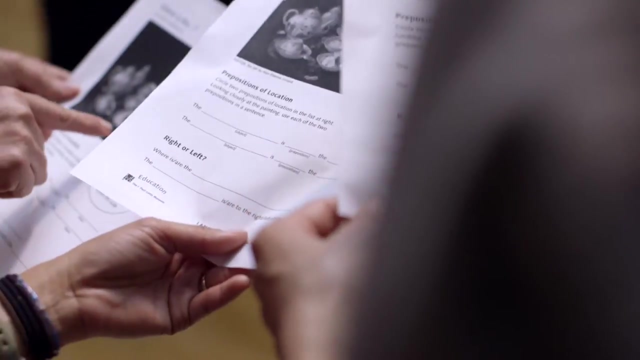 next to the bread. So I would like for you all to take turns. just sharing Next. all we wanted them to do was talk to their partners about the artwork. The teacup is on top of the saucer, The food is in. 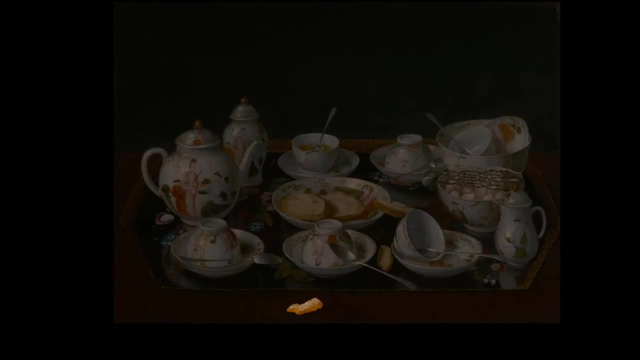 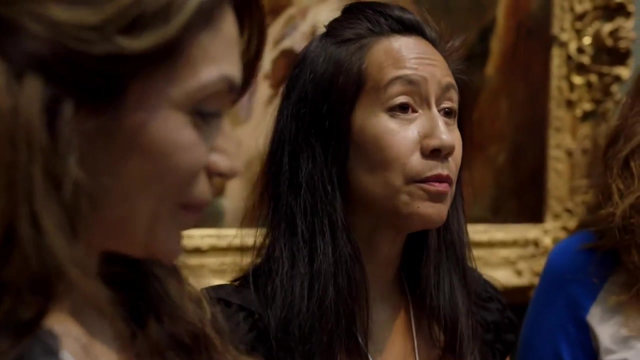 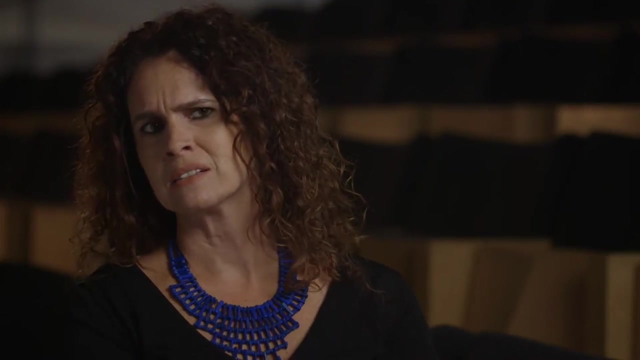 front of the lone, little food is in front of the tray. EL learners: they need to talk and hear the models as well. Other children may teach them. Oh, this is how you say it, So it's important to have that talking going on in class. The next step: 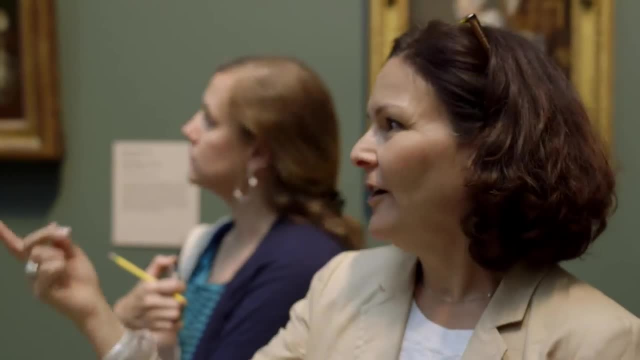 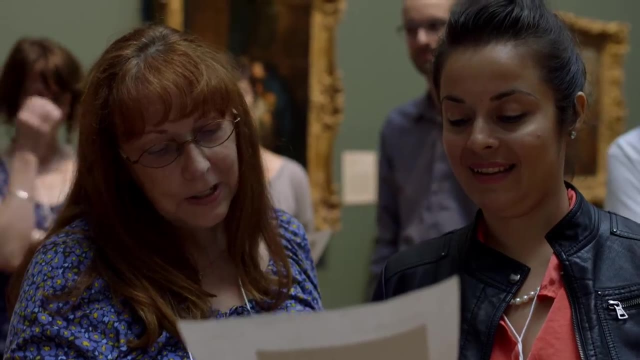 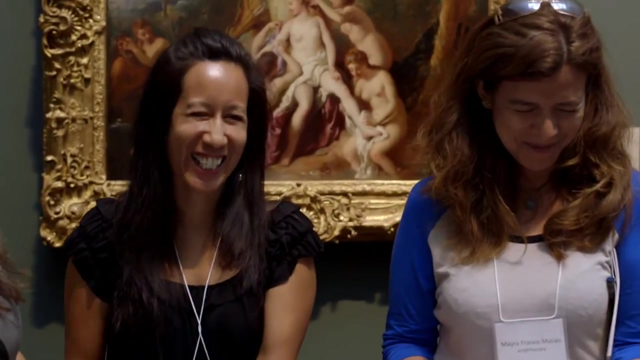 after that would be writing it out. But in the PD we really didn't get into that. We had the participants share what their partner came up with. The creamer is next to the teaspoon and sugar cubes. Anyone else The piece of food is outside of the tray. After that there were some other ideas. 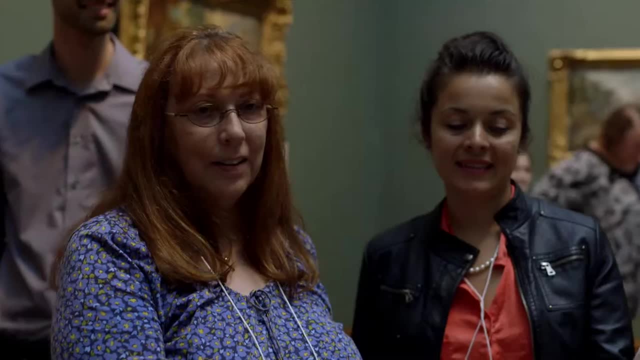 that we're formulating: Oh, I would do this, I would do that, I would do that, I would do that. I would do this in my classroom. Oh, I would do that. I think I'd actually have the prepositions on. 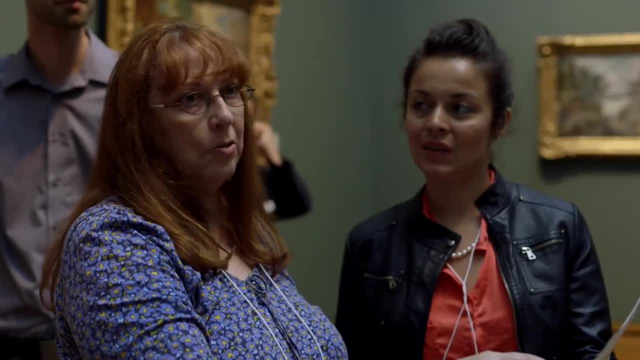 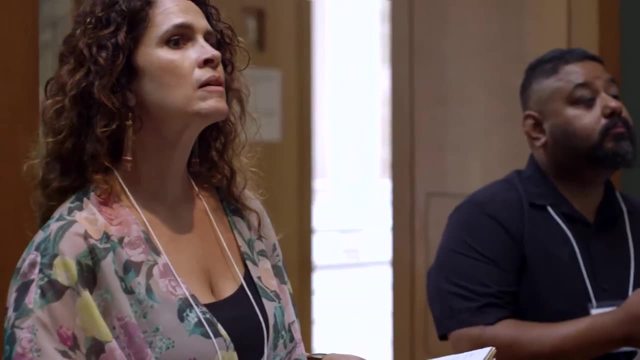 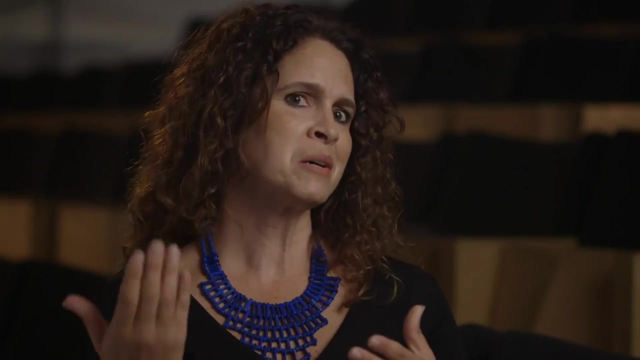 cards They could place them, see what next two looks like, and behind, because this is really tough for my students. It was great listening to the ideas that the teachers gave One little lesson about prepositions, how they would expand on it- Just hearing a couple of teachers talking about it. 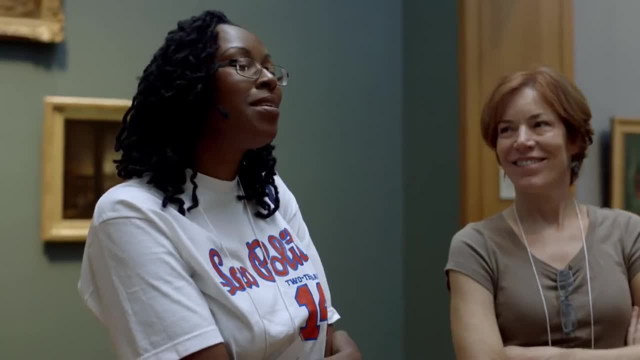 I thought, oh wow, I'm going to do this when I get back to school. Pamela and I were saying for older students as an example: I'm going to do this when I get back to school, I'm going to do this. 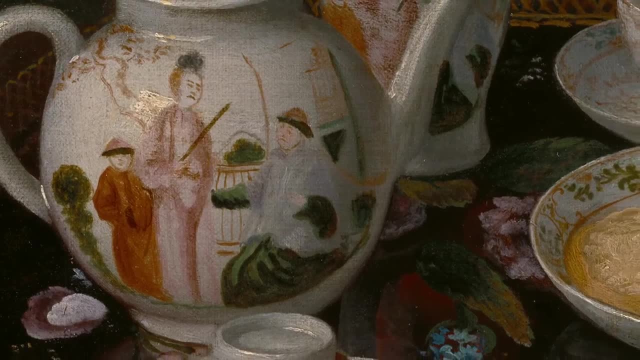 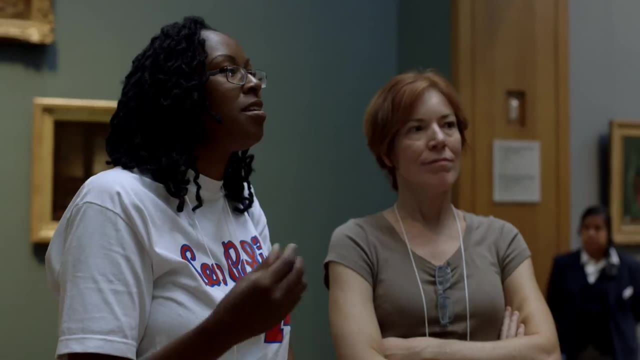 when I'm a student, and if not, I'm going to do this at an extension and you can get into social studies and how the tea set's seemed to have an Asian influence but the food seems European and so expansionism and trade and what was popular during that time, Yeah, and on this sheet it.